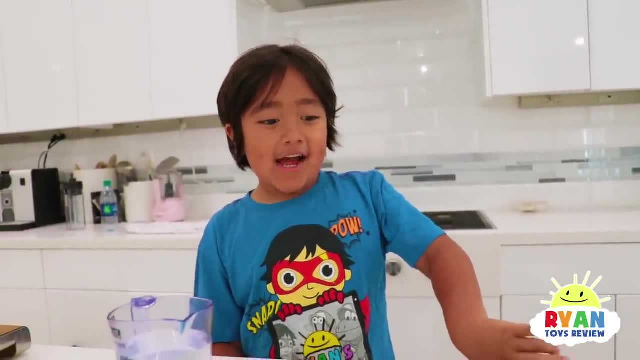 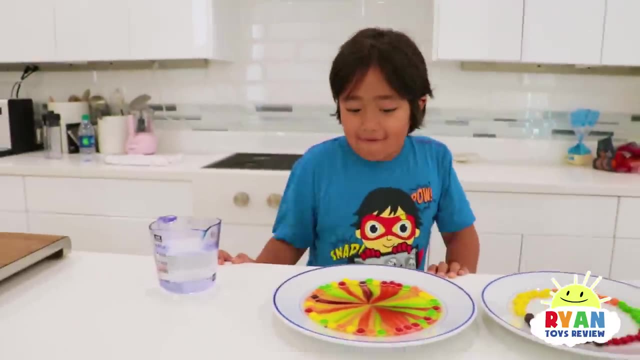 And what did you notice? Is the color mixed together? No, Look, it's separated right. All the colors did not mix, only meet in the middle. Now let's try the other one and see what it looks like. I think those colors are going to be really, really big. 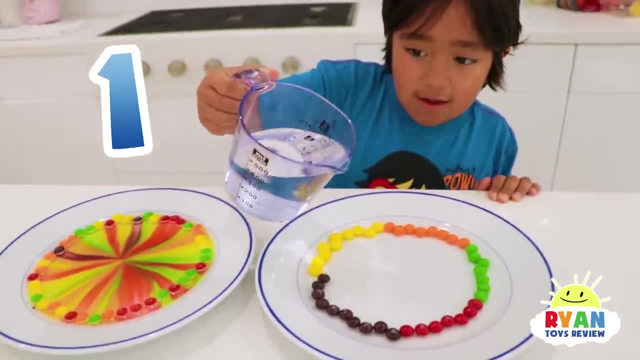 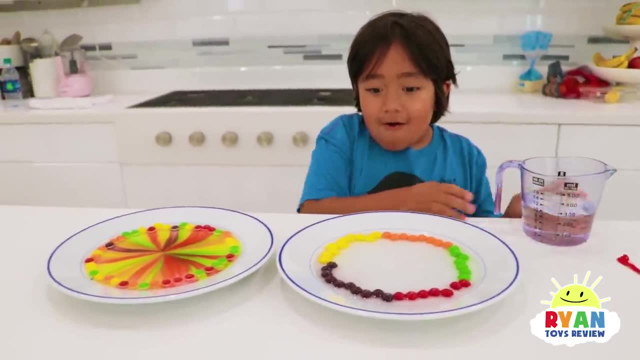 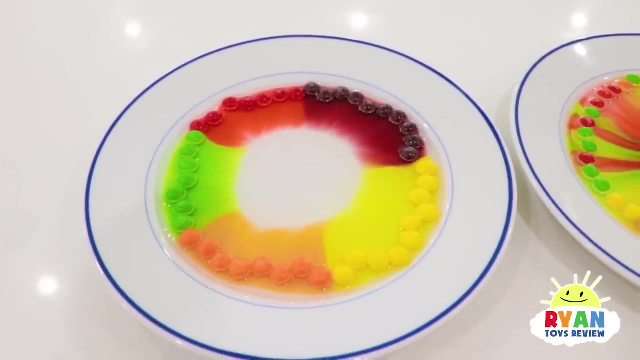 Three, two, one, That's enough. Whoa, What's happening? Whoa, You know, there's like a little toy thingy where it says: press this color, press this color, and then you have to follow it. 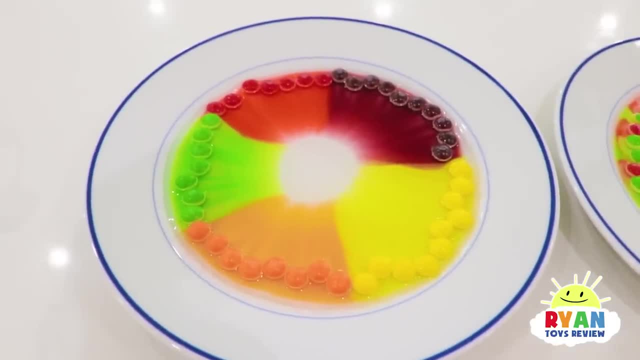 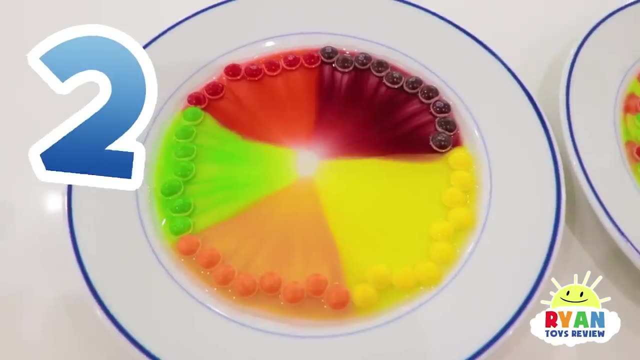 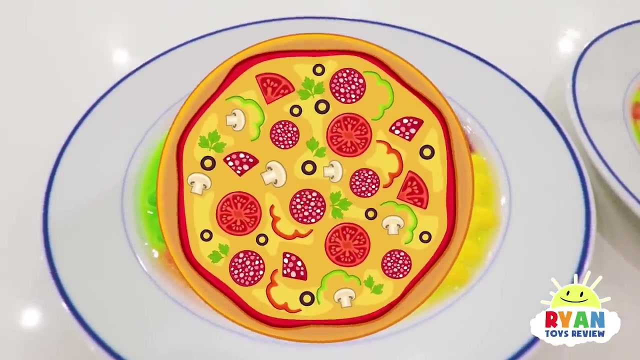 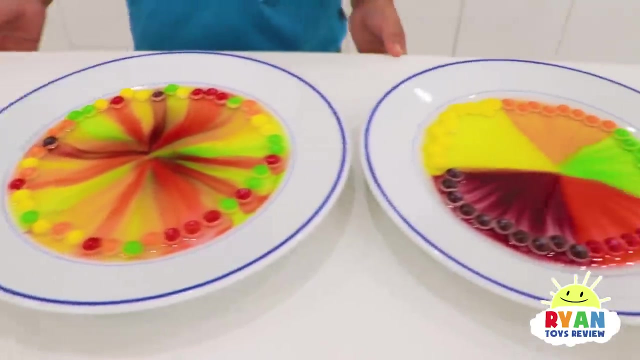 It kind of looks like that: Oh yeah, it does. Whoa, Three, Two, One, Five, Whoa guys, Whoa, That looks like a pizza, It does. It looks so cool, guys, It does. And look, since we did different patterns, they look differently. 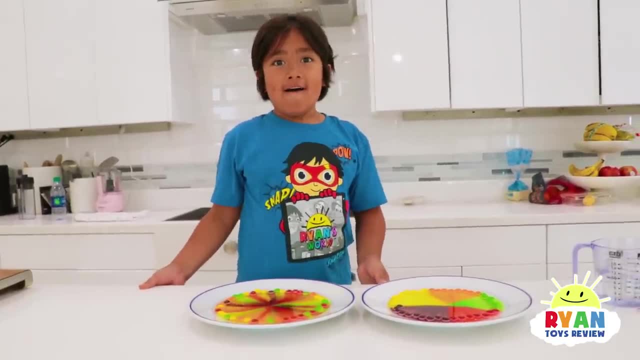 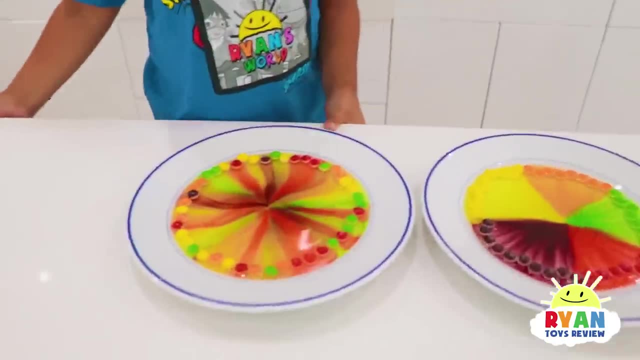 The question was: did the Skittles colors dissolve in water? Yeah, It did. yeah, The food coloring on the Skittles and the sugar both dissolve in water. That's how we get really cool colors like those. Hmm, If Skittles dissolve in water. 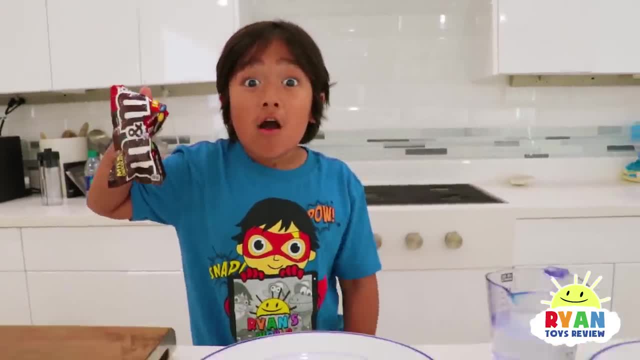 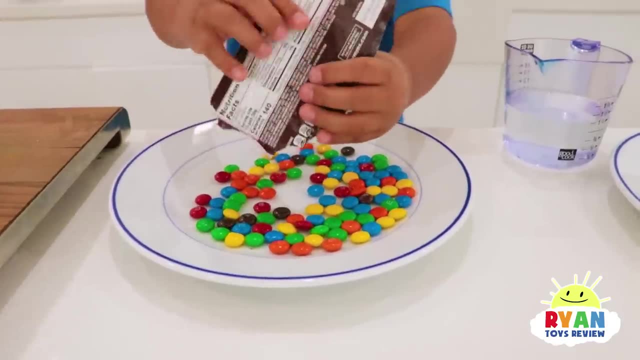 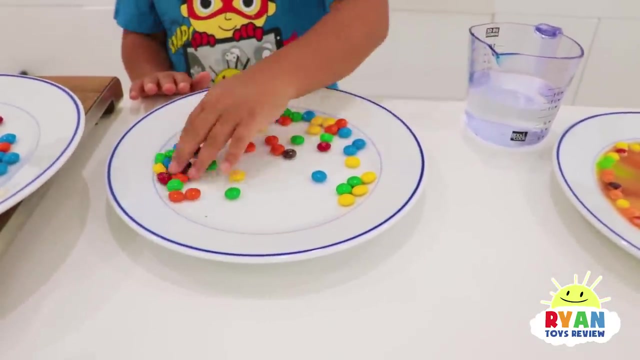 do M&M's dissolve in water? Find out? Whoa, Whoa. that's so much M&M's Now let's spread them out on the plate Like this. Let me make some of them big. Now I have two of them again. 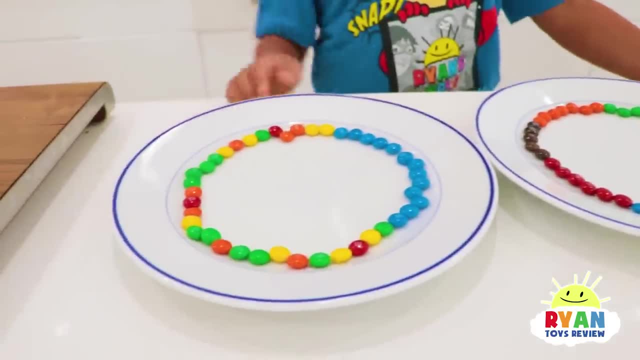 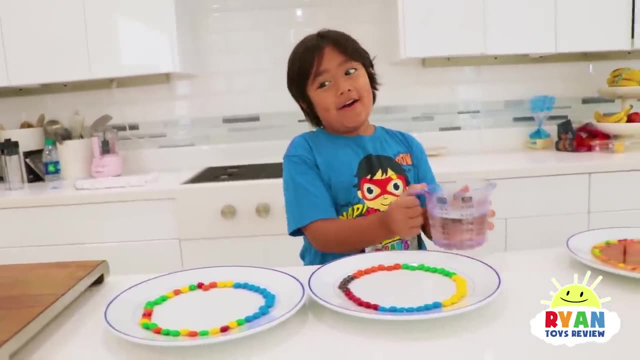 I have one with a lot of colors and I have one that's random. Let's try. So we're also using warm water. So we're going to try one with warm water and one with cold water. Let's see if it makes a difference. 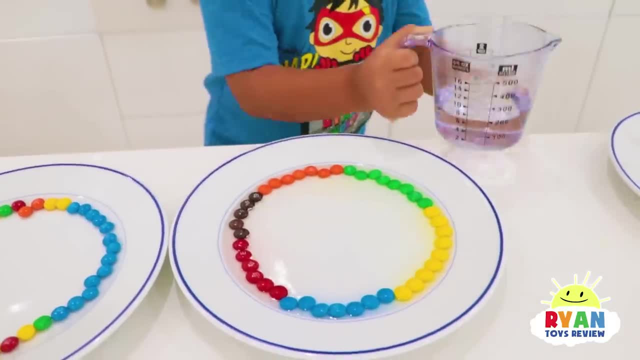 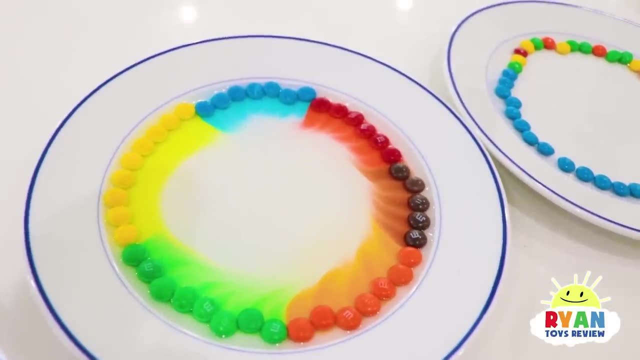 Warm water right here Starting. Is it working? Yeah, it is, Whoa. Yeah, so this is the M&M's. Do you guys see any difference between the M&M's and the Skittles? Yeah, the M&M's like twist. 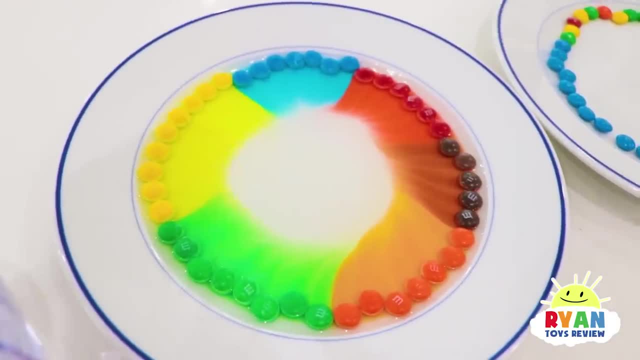 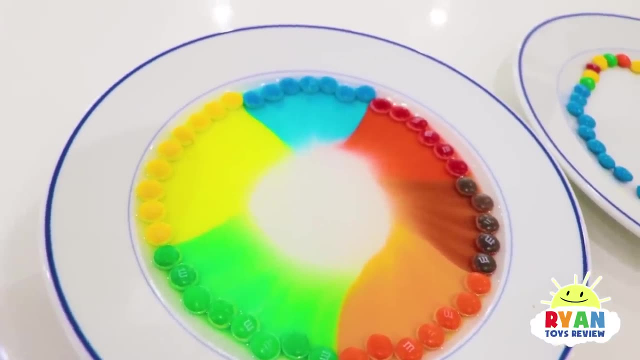 It looks so cool. Oh, Do you feel like it's the same speed or do you feel like it's different? Do you feel like it's different speed? It's different speed. So you think it was going slower than the Skittles or faster than the Skittles? 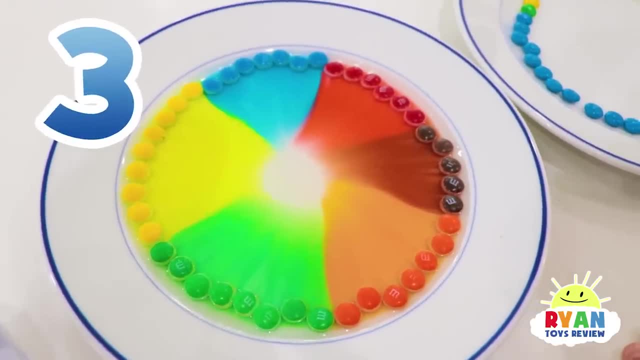 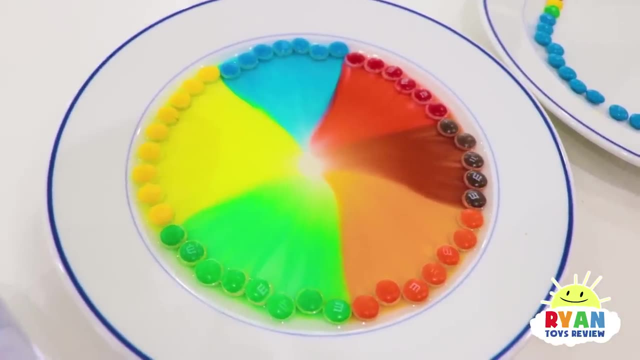 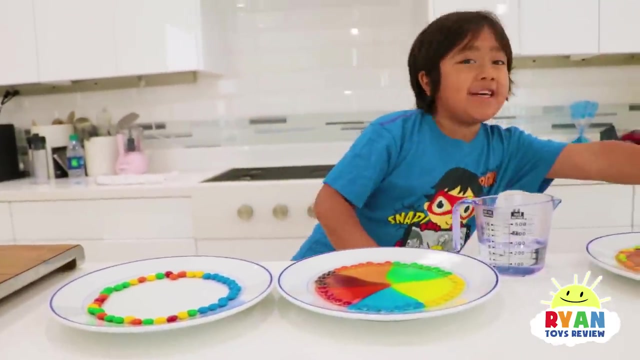 I think faster than the Skittles. Three, two, one, Bye, bye. There you go, guys M&M's. Which one do you like better, the M&M's or the Skittle one? So we've been letting these sit out for a while, so it looks super different. 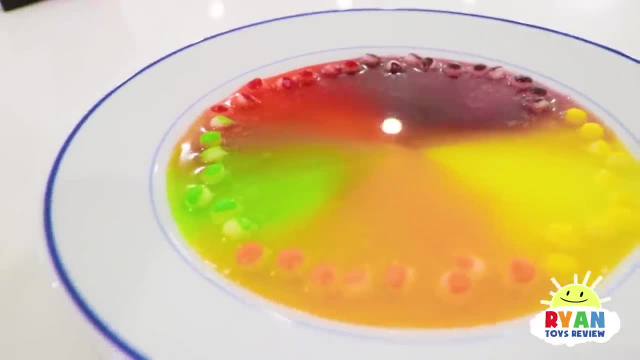 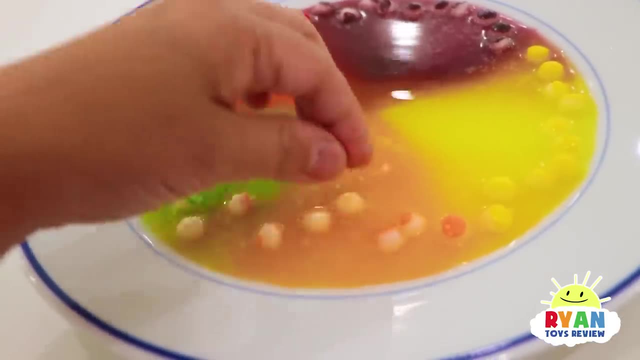 Everything is coming together there And here. if you guys look, it's all the little M&M pieces on the back. It's all white now. so, instead of the color, they're all white, Do you see? Because all the colors are coming out. 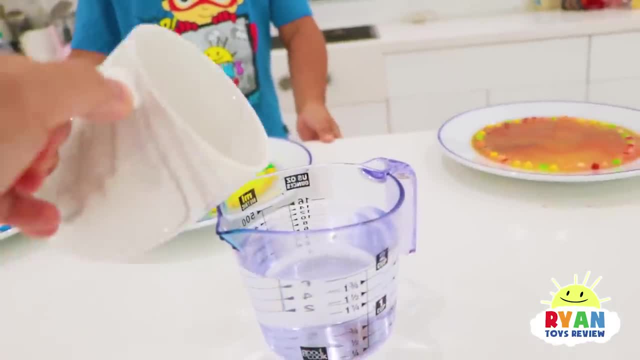 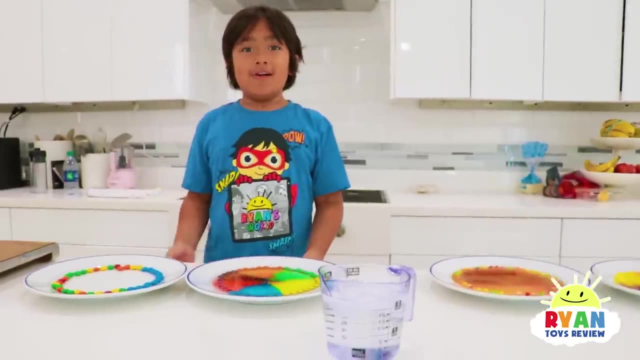 We got regular water for the sink and now we're going to add ice to it to make it ice cold. Ooh, We're going to let it wait for like one minute. That's right, Ryan, to make the water cold, yeah. 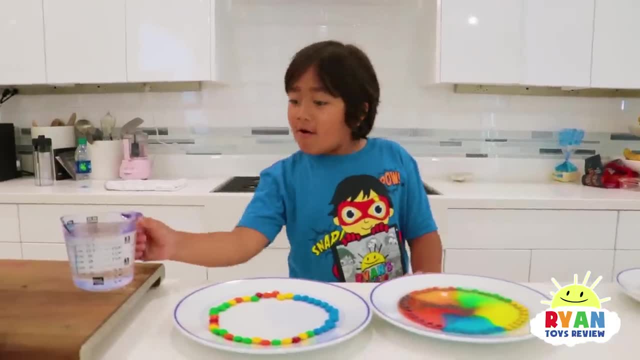 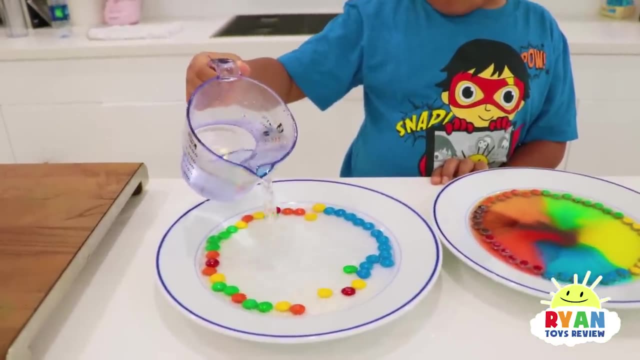 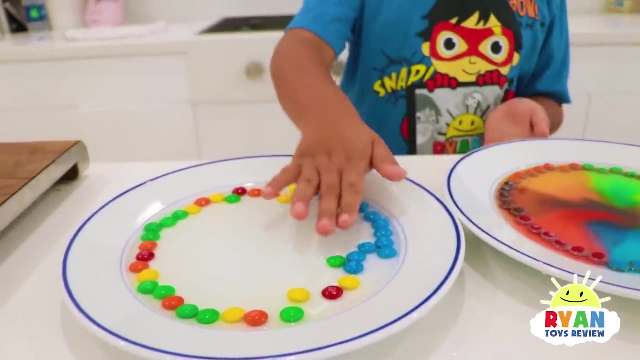 Ooh, Okay, I think it's ice cold now. Oh, Three, two, one. While we wait, do you guys think it's going to dissolve? Good question, Ryan. What do you think? Do you think the cold water or the hot water will help it dissolve faster? 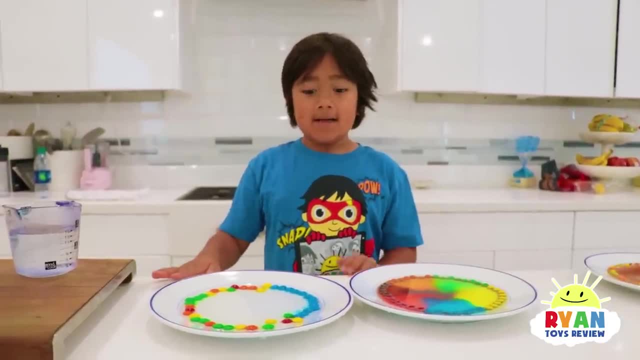 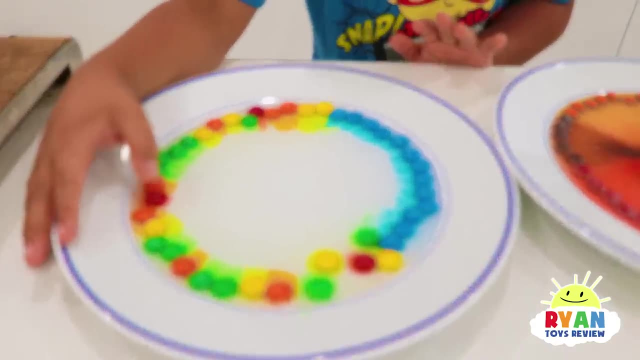 I think the hot water will dissolve faster. Okay, let's check it out and see. So we're going to have to wait. It's working Well. if you move it, it goes faster. We're going to wait and see what happens. 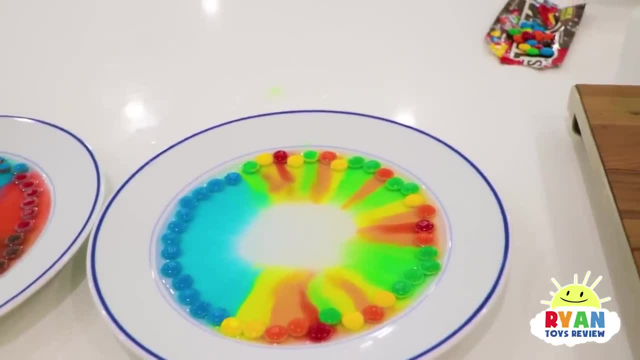 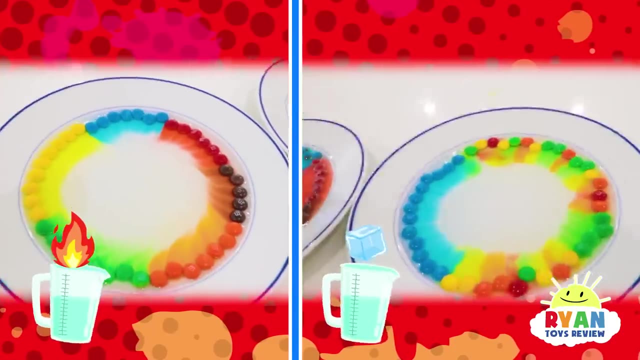 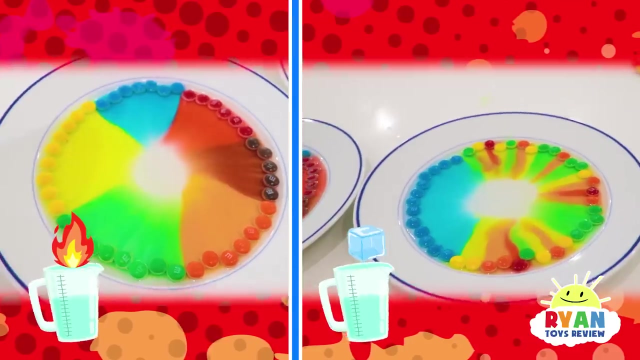 There's the cold water. as you notice, I think it's going a lot slower. Yeah, So we're waiting for a while now. It's still working. Yeah, It's just not going as fast. Wait, We're waiting. 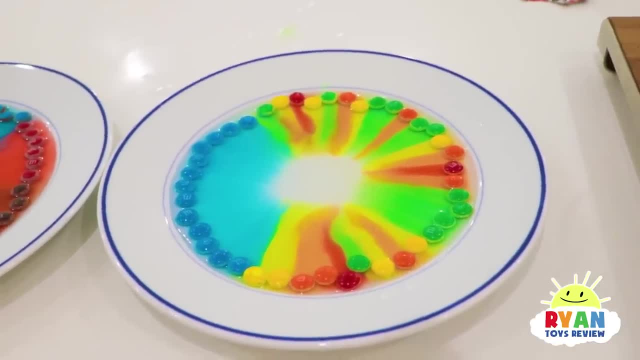 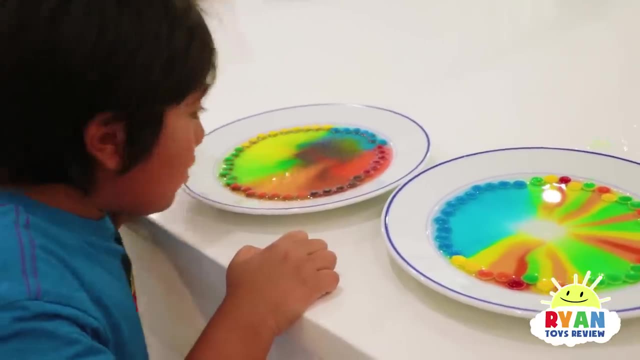 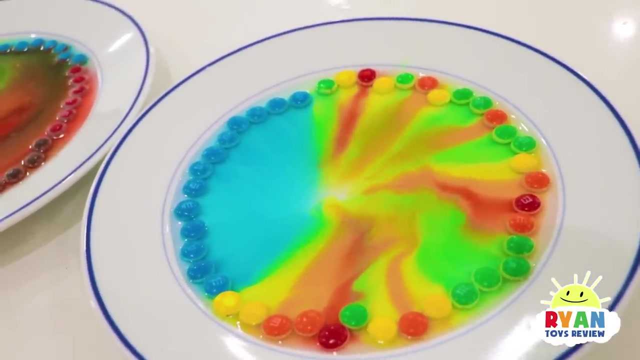 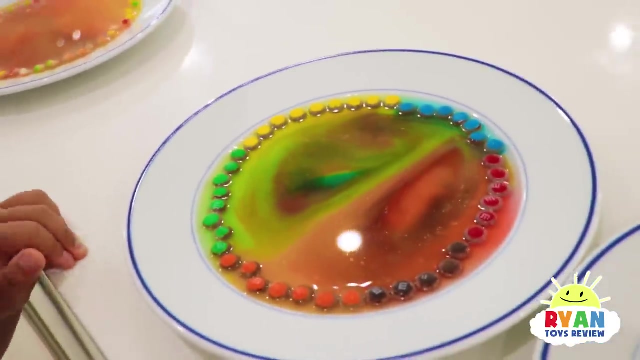 What happens? if you like, blow it, Oh, great question. Why don't you do it? Oh, it doesn't change it, It just changed the water. Okay, Wow, it's mixing it all together. Whoa, it's creating like a galaxy color.